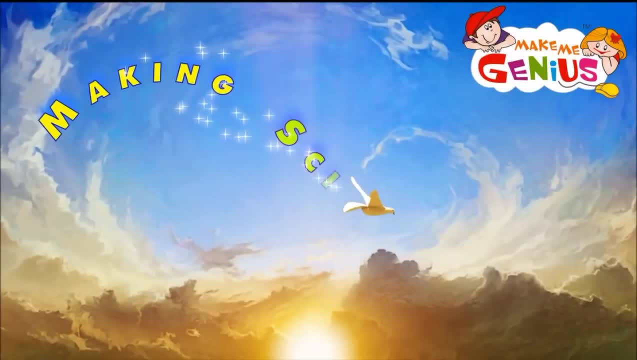 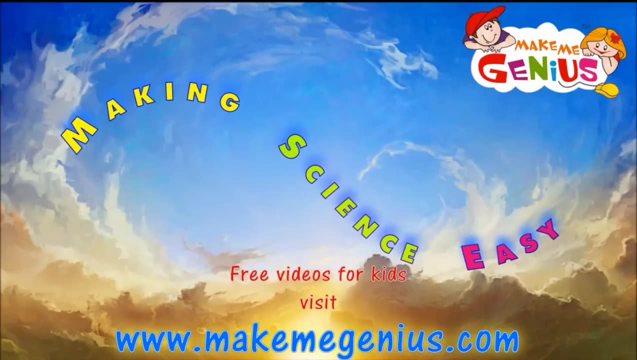 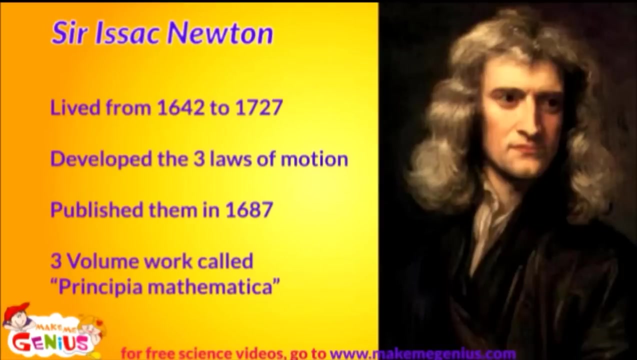 Did you know that physics is about how things move and why things move? It was Isaac Newton who discovered the three laws of motion. He was a scientist who lived from 1642 to 1727.. Let's first learn about the first law of motion. 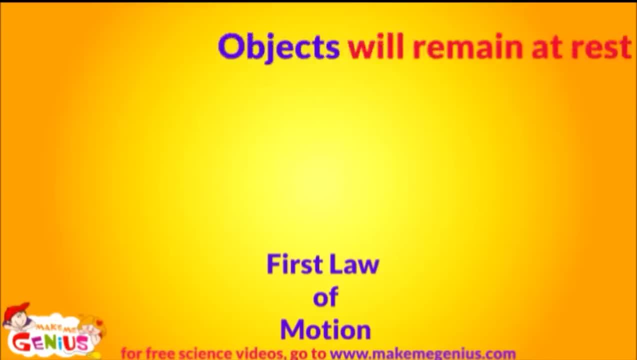 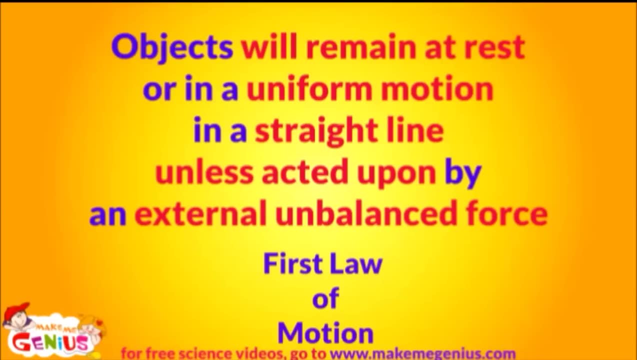 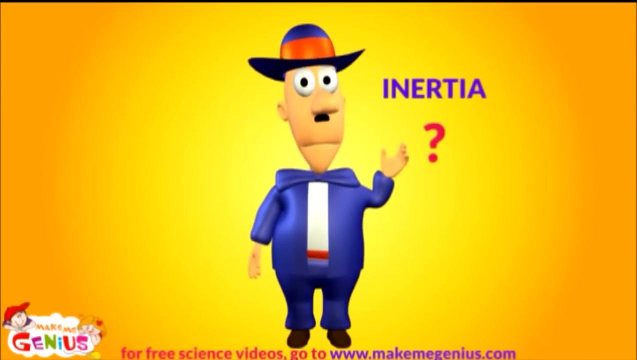 It is also called the law of inertia. It states objects will remain at rest or in uniform motion in a straight line unless acted upon by an external unbalanced force. To understand Newton's first law completely, we need to learn about inertia first. See, this is a very large sofa. 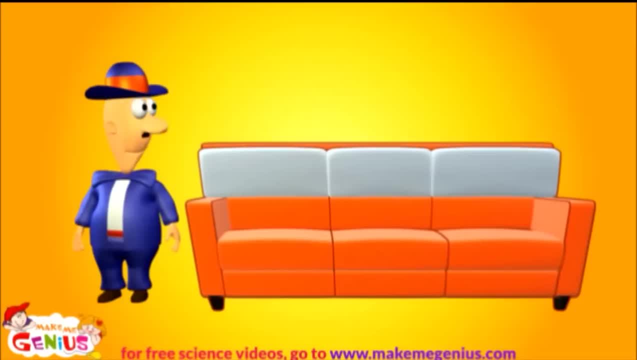 What's special about it? It's stable. It is not moving. Now go ahead and try to move it. Oh, you can't, It's not willing to move. You can't move it as it is very large. Now try to move this small stone. 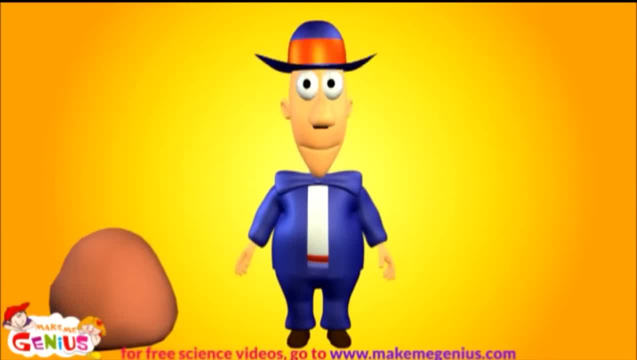 Good, You can move it a little bit, but you had to put in a lot of effort. It was also like it didn't want to move from its original position. Even the smaller things don't want to change their positions. They don't want to move. 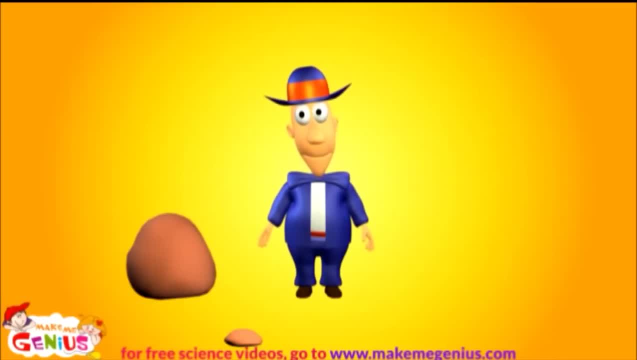 Even a small stone takes some effort to move. This is the first rule of physics. Things like to stay where they are. No object in this universe would start moving unless some external effort is put on it. It's like all things in the world are lazy. 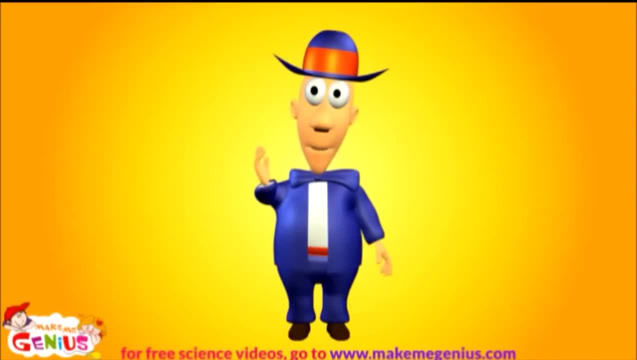 Now the question is: if things are lazy and they don't want to move, then how does the movement happen? The answer is that there are so many things in the universe which push and pull other things and force them to shift their positions, like you forced the small stone to move. 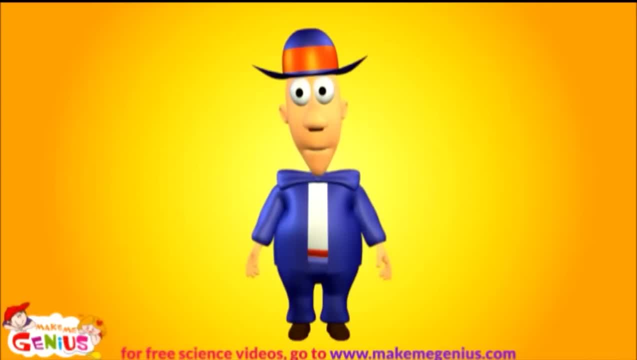 But, as we said earlier that things are lazy, they would try and stop their movement as soon as the effort was removed. Well, you'll be wrong if you think like that. You'd find it very strange to accept that when a small stone was still, it wanted to stay still. 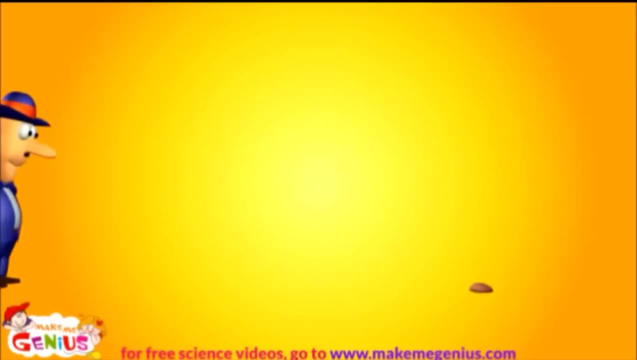 And once you'd put it in motion, after putting some effort, it would like to keep on moving. In reality, it would keep on moving forever and ever, But somehow it stops. But it stops not because it wants to stop. It stops moving because things in its path force it to stop.